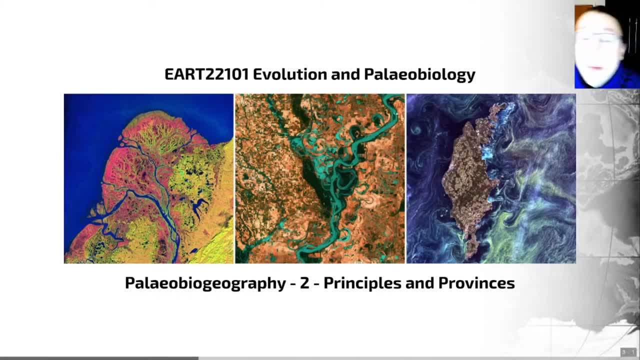 And welcome to video number two of Paleo-Biogeography, in which we're going to be looking at some of the principles of paleo-biogeography, so defining some terms, and then we'll finish by looking at some things called biogeographic provinces and look at how these change over deep time. 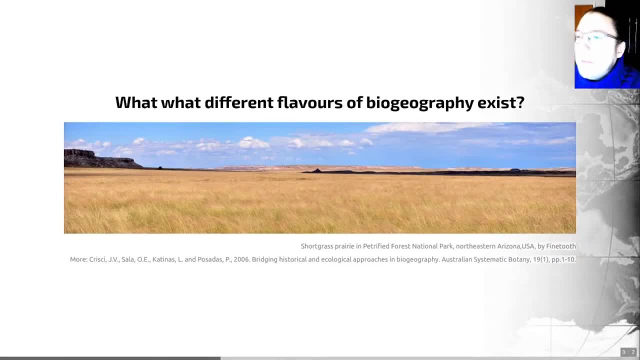 So let's start off by looking at some of the different flavours of biogeography that exist, so the kind of different ways we can divide the fields to make it easier to understand. So I think the first useful division to make is to highlight that biogeography can both be descriptive, so this is describing and recognising patterns in the distribution of species. 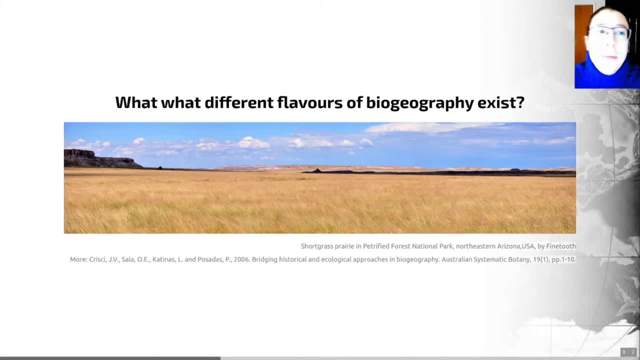 or it can be interpretive. so this actually tries to explain those patterns, so it looks for causal explanations of species distributions. Studies in the latter form, interpretive biogeography, where we're actually trying to explain the distribution patterns of species distributions, can then be themselves split into two kind of categories, and these categories are either ecological or historical biogeography. 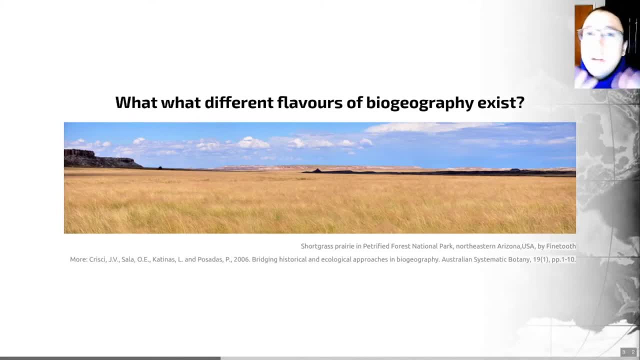 And really the difference between these two kind of types of interpretive biogeography are just the scales that they look at. So ecological biogeography searches for causal explanations of the distribution patterns at short temporal and spatial scales. so we're looking at limited time frames on, for example, a continental or smaller scale. 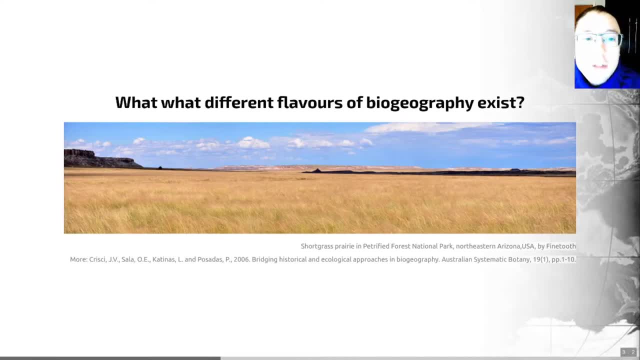 In contrast to that, historical biogeography concerns more evolutionary processes that may occur over millions of years and will occur on the scales of kind of continents. This is a difference that's illustrated by the realisation or the recognition that two locations in the world with very similar abiotic characteristics, such as 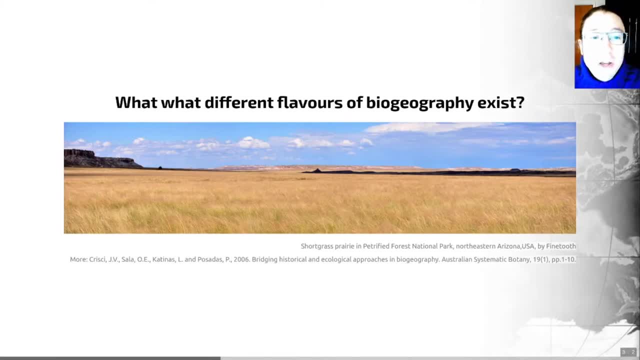 temperature and precipitation, may have identical functional groups of organisms in them and they may be very considered, very similar from an ecological point of view. so that's the ecological perspective. However, they may have quite a different species composition. so the species that actually make up those different 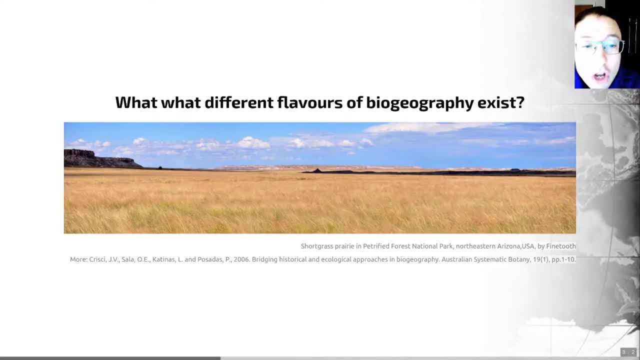 animal communities and that take on individual roles could be radically different, and this marks the difference between ecological and historical biogeography. I thought it would be useful to have a very quick example to illustrate this. So, looking at climatic conditions in the temperate, arid and semi-arid regions of North and South America respectively. 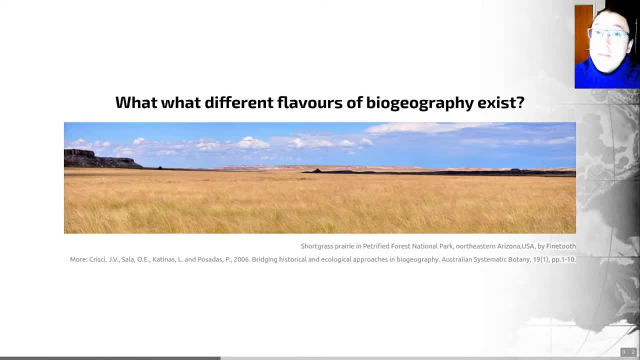 the conditions here are quite similar, So actually from an ecological point of view, these ecosystems look relatively similar. However, in the North American steppes and prairies like the one that I show in the image here, we know that these plants have evolved under intensive grazing, from bison, for example, while equivalent taxa, so large members of this group that bison belong to, called the ungulates were. 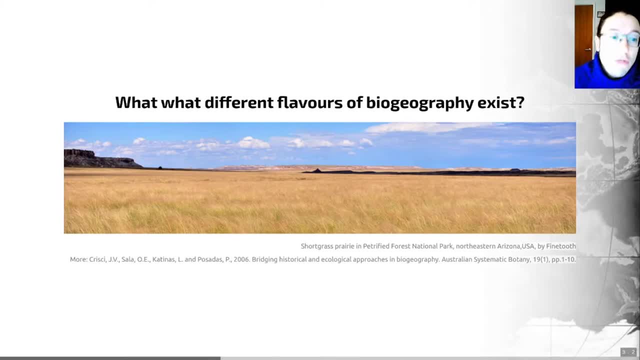 ambescent from South America at the time when these grasslands evolved. So if we're thinking about this within the kind of framework of ecological and historical biogeography, ecological biogeography on its own can't account for that lack of ungulates in South America. 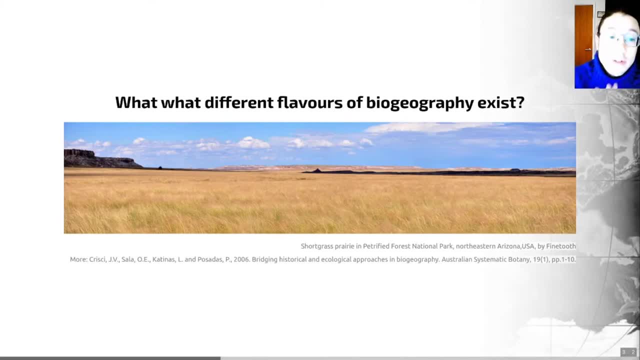 That is to do with the configuration of continents in deep time, But also historical biogeography on its own can't explain the nature of the arid and semi-arid vegetation that we get in Central North America That has evolved in concert with the bison. 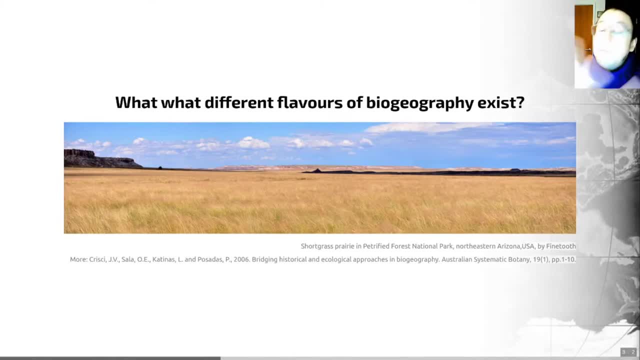 And so these two concepts are quite strongly linked. They need each other to explain the patterns of biogeography as fully as we would like to be able to Bear in mind. of course, since this lecture is focusing on paleo-biogeography, we'll be more thinking along the lines of historical rather than ecological biogeography much of the time. 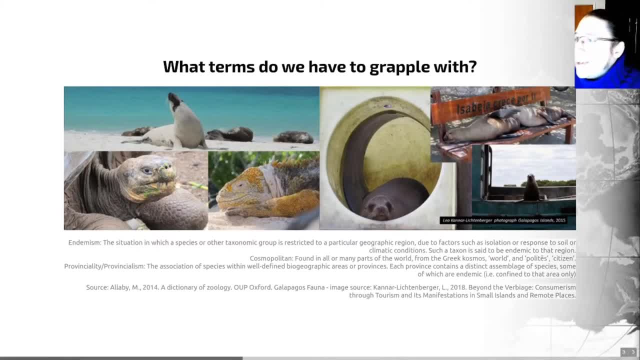 As part of this introduction to the area I also wanted to talk about- sorry, I wanted to define some terms for us, So here we go. Let's define some key terms. An endemic species is one that is local or regional, and the property of being endemic is called endemism. 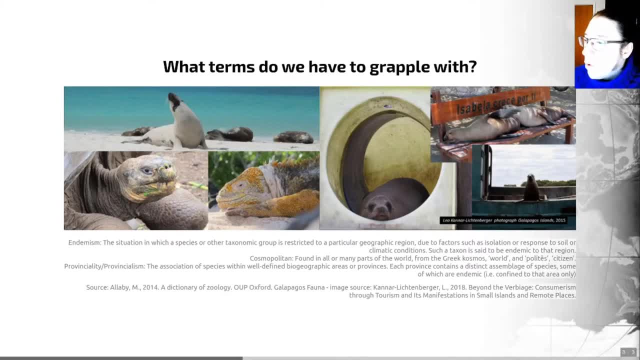 That makes sense, Right? So I've put a definition of endemism on the slide for you. Endemism is the situation in which a species or other taxonomic group is restricted to a particular geographic region due to factors such as isolation or response to soil or climatic conditions. 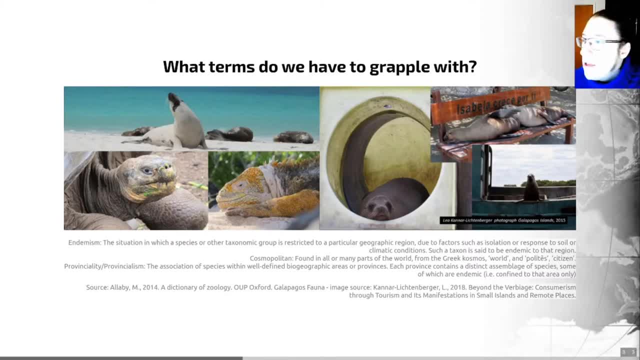 OK, so, for example, all of these species that are shown here are endemic to the Galapagos Islands, So they are found only there in many cases. A contrast to that is the idea Of cosmopolitanism. So a cosmopolitan species, one with a cosmopolitan distribution, is one which is widespread. 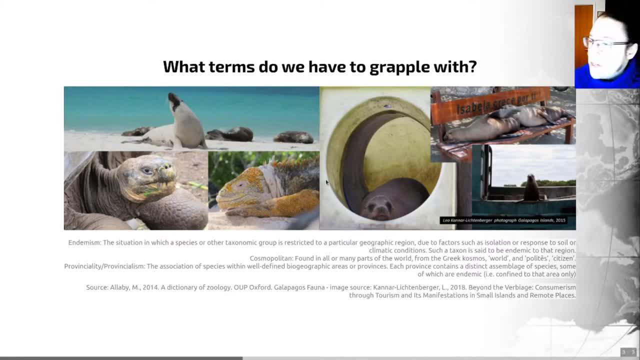 So the definition I've put on the slide here says it's a species that's found in many or all parts of the world, from the Greek cosmos world and polites citizen. So that's cosmopolitanism. Be aware that sometimes you may come across the term pandemic, referring to a distribution that's 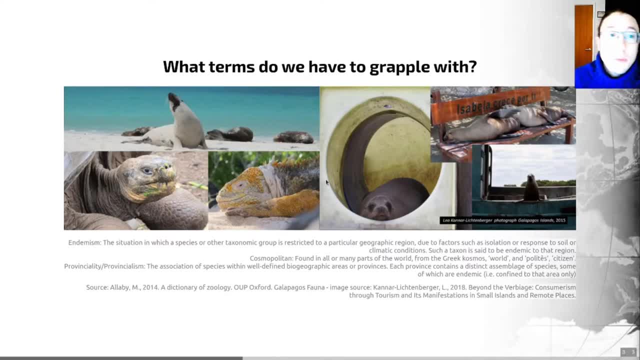 somewhere in between these, or overlaps with cosmopolitanism. This is often avoided as a term due to the obvious overlap with epidemiological topics. So, for example, we're suffering from a pandemic right now, but also it has a relatively poor definition. 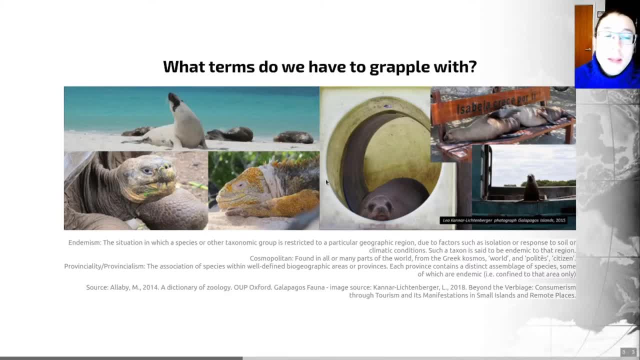 So some consider pandemism to be between endemism and cosmopolitanism, So widespread, but with a few gaps. And there's this. this term has suffered from inconsistent usage, So I wanted to highlight that it exists, But then I also wanted to say that I won't be using it much further today. 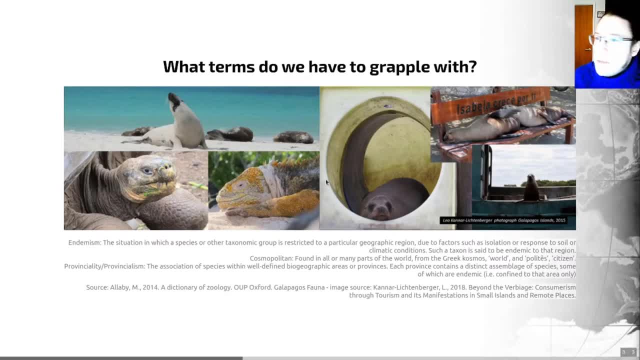 Bear in mind also that endemic species, so these species that have distinct geographic ranges, rarely occur in isolation, Where they are found together. this is something that's called provincialism, So I'm going to be going into this further on the next slide. 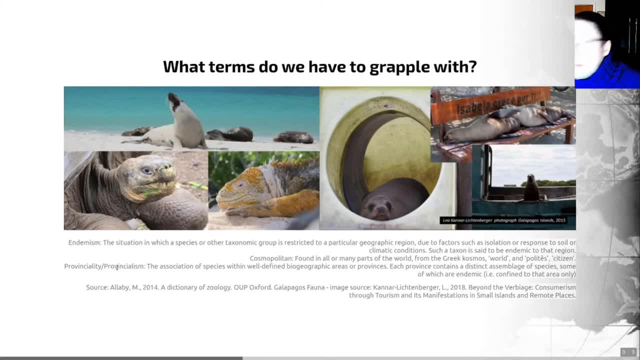 So provincialism or provinciality? I've seen both of them in use. I don't know if there is a correct answer, But this is the association of species within well-defined biogeographic areas or provinces. Each province contains a distinctive assemblage of species, some of which are endemic. 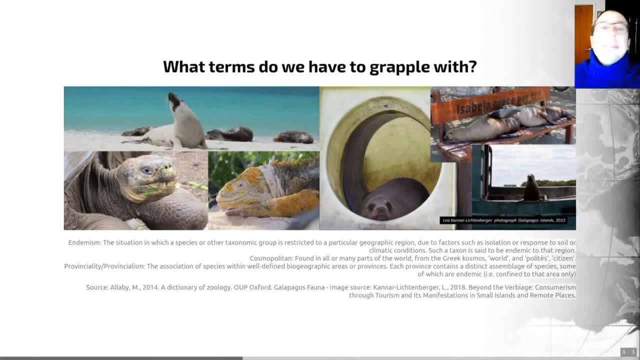 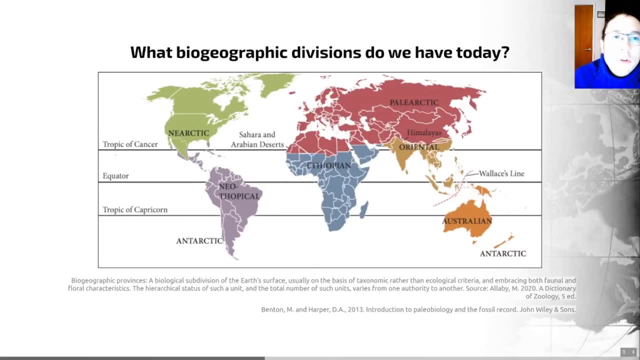 So confined to that area only. So this is kind of like a step up. from a single species is the collection of species when in a particular area. So this idea of provincialism reflects a useful concept, And that concept Is the biogeographic province. 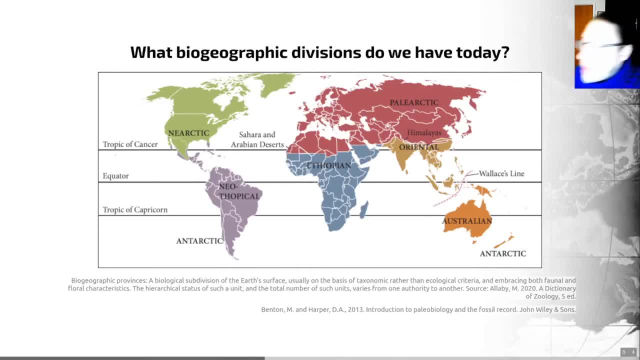 So I've put a definition of this term on the slide for you as well here. A biogeographic province is a biological subdivision of the Earth's surface, usually on the basis of taxonomic rather than ecological criteria. It embraces both formal and floral characteristics. 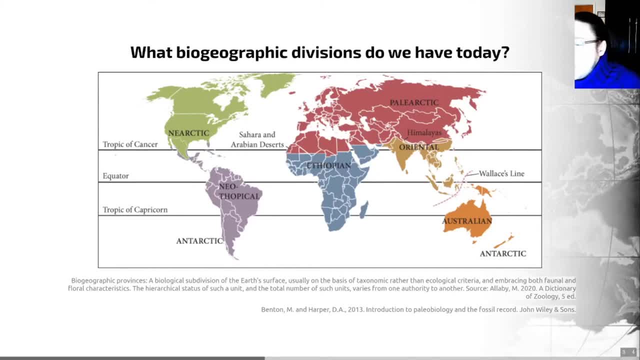 The hierarchical status of such a unit and the total number of such units varies from one authority to the other. But you can see to illustrate this on the slide. I've put a definition of this term on the slide for you as well. here I've put one particular definition up, which is which divides the Earth today into six main biogeographic provinces that are labelled on this map for you here. 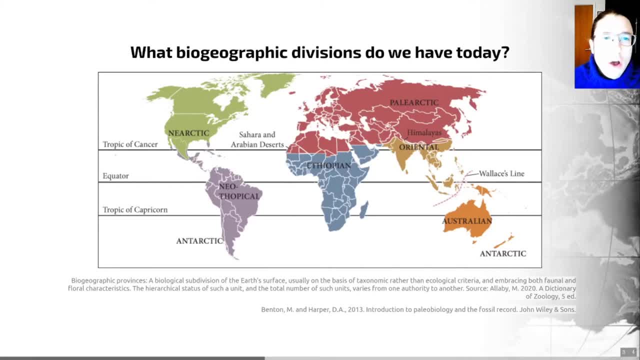 These particular provinces are based largely on the work of a scholar called Philip Sclater. as, along with Alfred Russell Wallace in the late 1800s, So provinces are characterised by their endemic species, which have restricted ranges in contrast to cosmopolitan. 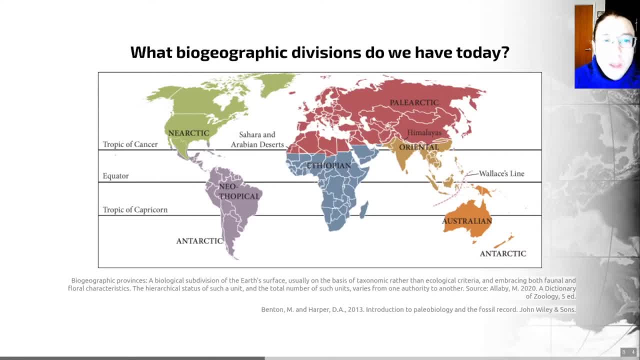 So that's how we define our provinces, But I want you to bear in mind, before I move on, that this is just one of a number of schemes that are used to define biogeographic regions, And these schemes are often based around different things. 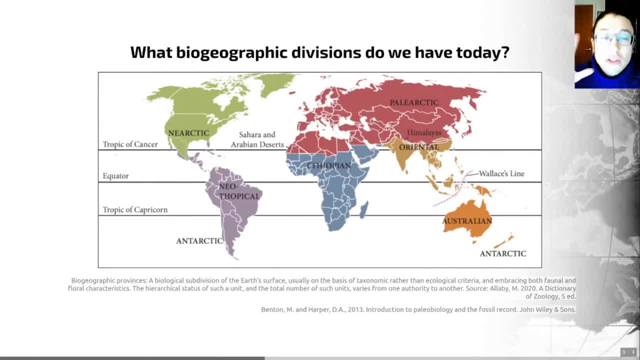 It could be species composition, such as our definition here, But there are a whole host of other ways of dividing up the world into, for example, different ecological zones which are different from the definition I've given you on the slide. So other biogeographic units that are used in other schemes include biogeographic realms. 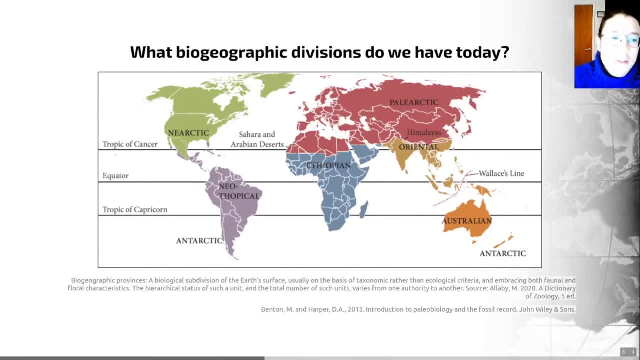 or sometimes these are called ecozones, bioregions, floristic regions, ecoregions or zoogeographical regions. So these are all different ways or different concepts we can use to partition space in the real world. So just be aware that those other definitions do exist. 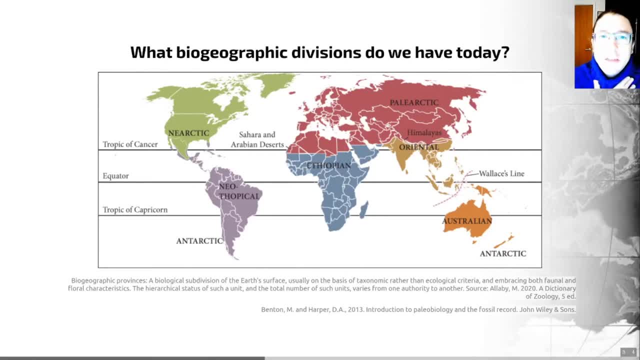 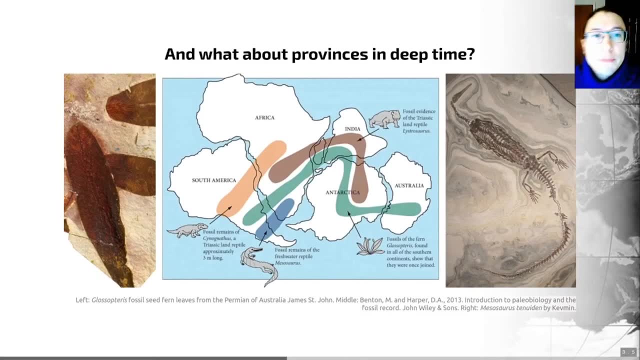 But for our purposes today, I think biogeographic provinces is a very useful definition, And it's one that we'll be using throughout the rest of this lecture. when I'm talking about these divisions, Bear in mind also that biogeographic provinces existed in the past as well. 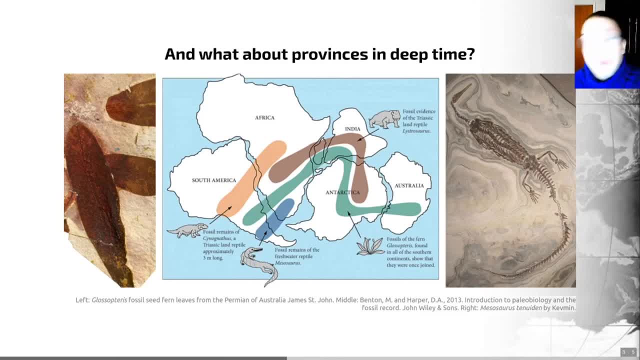 I put this video in the last, sorry, I put this video. I put this image in the last video to demonstrate that fossils in deep time are like, are key to kind of building a clear picture of the distribution of continents. What's this diagram actually doing? 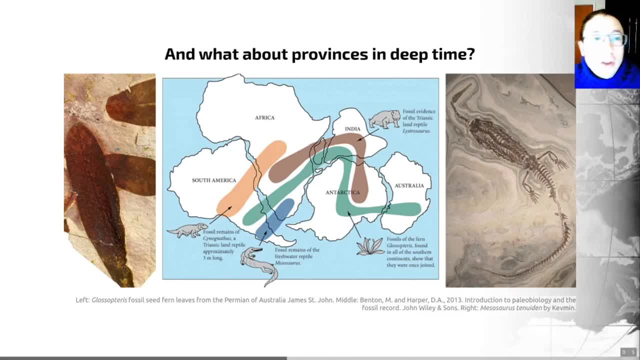 It shows- and I kind of glossed over it last time- is the Carboniferous and Permian distribution of taxa of a range of different species and genera, including the Glossopteris flora. An example of Glossopteris is shown on the left hand side here. 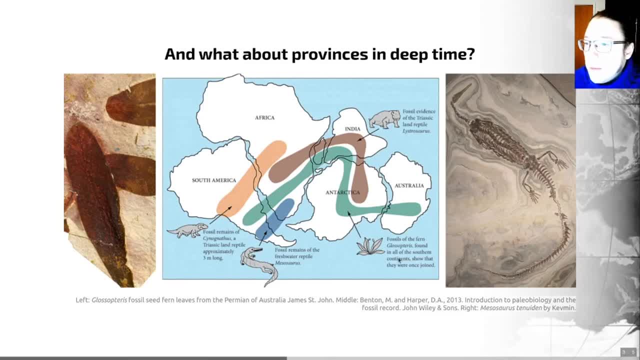 So this is known from fossils across the world And it's this green zone here along with the Mesasaurus fauna. This was a fresh water reptile shown on the right here, And this is the Mesasaurus fauna And this is represented by this blue blob here. 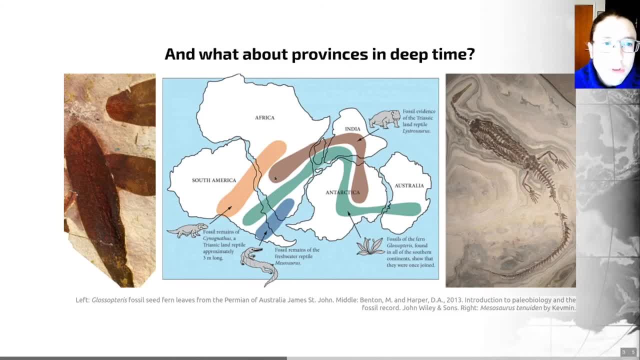 And there are a couple of other important species for our purposes here, And the correspondence of these fossil faunas and floras across the southern continents suggests- and did so to Wegener and others- that South America, Africa, India, Antarctica and Australia. 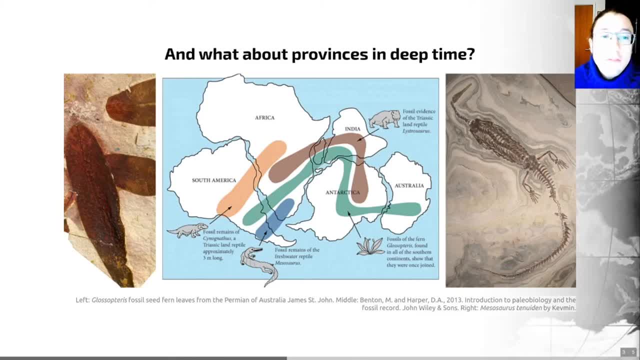 had all been a single continent at one point and have drifted apart since. More generally, provinces like this have been recognised throughout the Phanerozoic, both on land and in the sea, and in a great many different groups of organisms. So those are basic observations of the kind that can be made by hand. 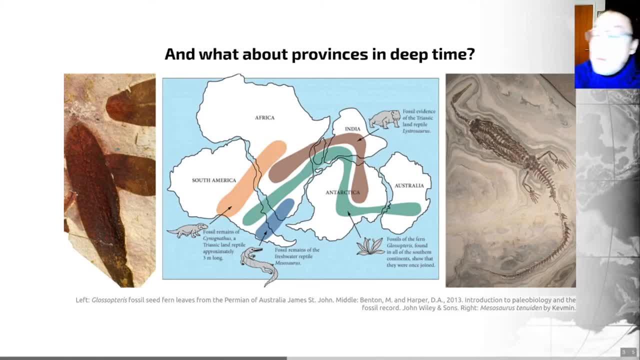 and indeed were for the purposes of the early debates on plate tectonics, for example, And these can now be supplemented using a computerised paleogeographic systems or GIS, to kind of better quantify the distribution of these different fossils. 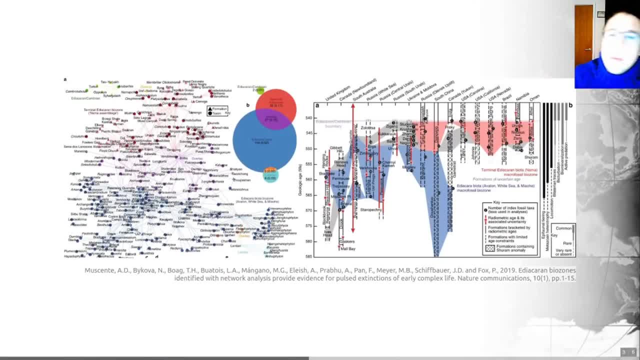 And I wanted to finish this video with a highlight kind of like, by highlighting the distribution of provinces through time. So just as plates- the Earth's tectonic plates- move through deep time, the positions, shapes and sizes of biogeographic provinces also vary. 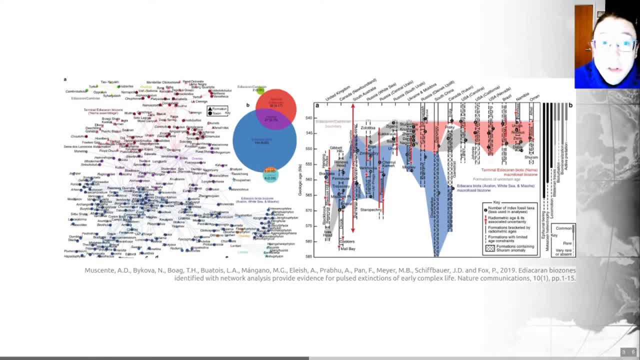 Barriers and migration routes come and go, climatic belts fluctuate with changes in climate and there is a turnover in animal communities associated with this as we look back into the deep geological past. So I'll provide a very quick whizz through how these change through time. 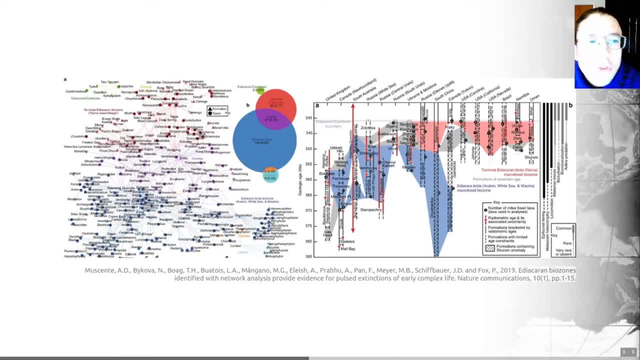 Now, these provinces in the Precambrian were dominated by microbes and they were very different from those provinces that we see today, which are defined by a great diversity of animals and plants, and indeed it's far harder to get a handle on what provinces may have looked like when we go. 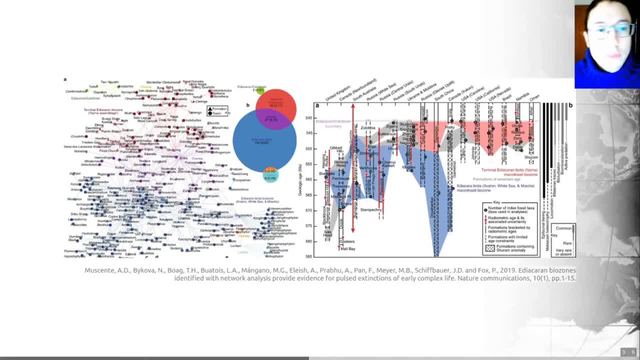 before the Precambrian period. There is some evidence in the late Precambrian that Ediacaran biota had some provinciality. In fact there's some really cool recent research. I've put a reference to the paper that I've used as a source for these images on this page here. 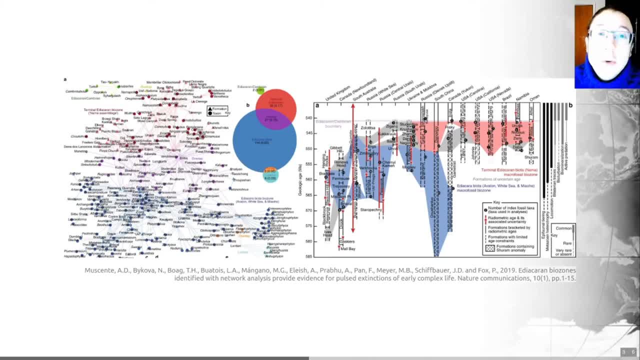 that has used a technique called network analysis to understand the distribution of Ediacaran taxa. There's a network, shown on the left here, which is just a collection of relationships in both space and time between different taxa, And through this analysis the authors have demonstrated that the Ediacaran system 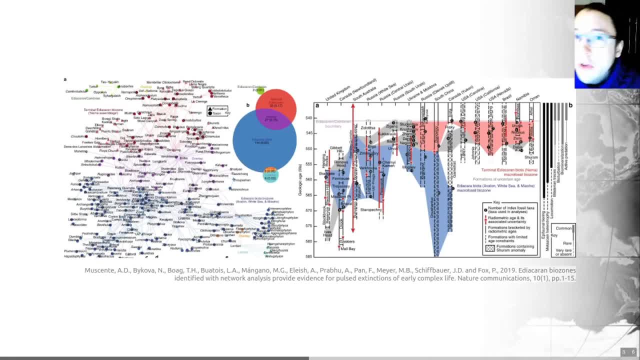 contained a number of environmental, ecological biotypes- So these are, I guess, an equivalent of our provinces- as well as a series of assemblage biozones. So these are time-based divisions that are shown in blue and red on the right-hand side. 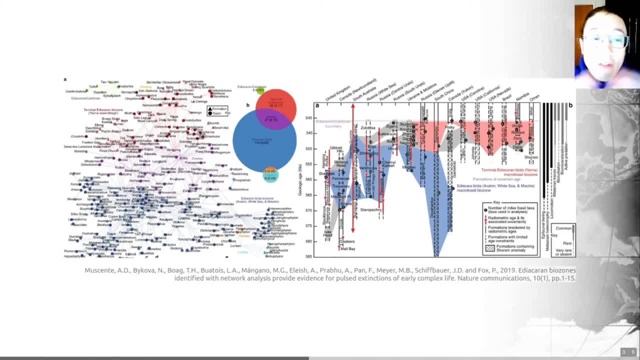 here. By doing this analysis and unraveling these two, the authors have managed to show evolutionary and ecological changes that led to the Ediacaran-Cambrian transition, as well as presenting evidence for extinction events at this time. So that's a really exciting piece of research. 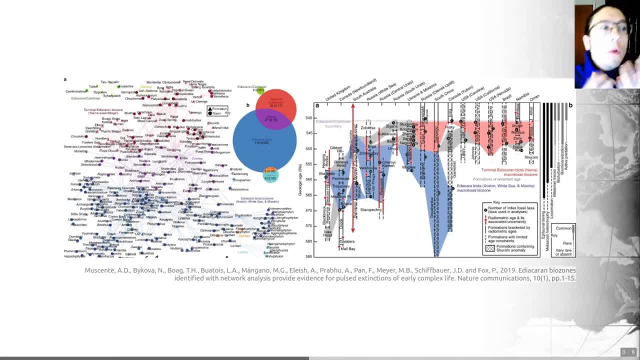 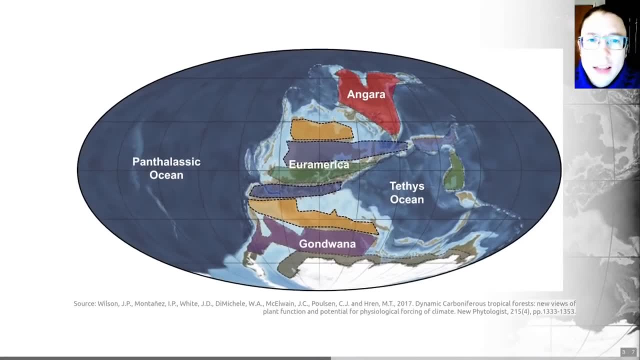 and a good example if you want to dig a tiny bit deeper into the more quantitative approaches that modern studies are using to understand paleobiogeography. So that's the late Ediacaran, which, for our purposes, is the first point at which we can see provinciality appearing. 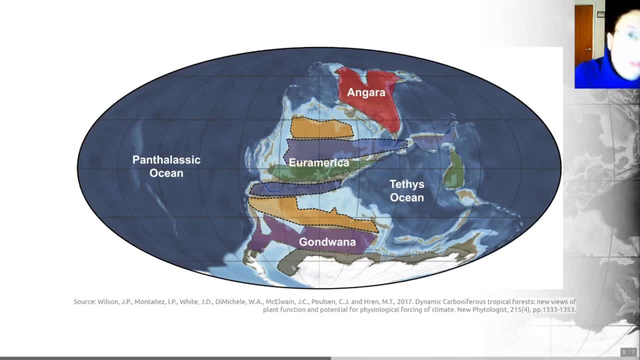 As we move into the Phanerozoic, so this is the Cambrian and onwards animal communities of the early Paleozoic were clearly grouped into biogeographic units. So, as an example, during the Cambrian and the Ordovician provincialism across most marine, 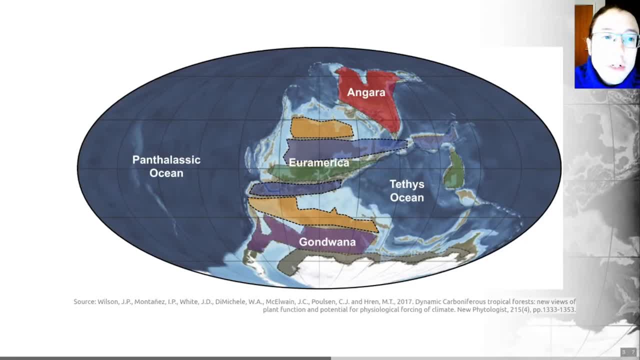 groups was fairly clear. It was well marked, And this is particularly true of the Brachiopods and the Trilobites. These are really, really useful to understand the history of the past continents. There was an interval of cosmopolitanism, so widespread species in the Silurian period. 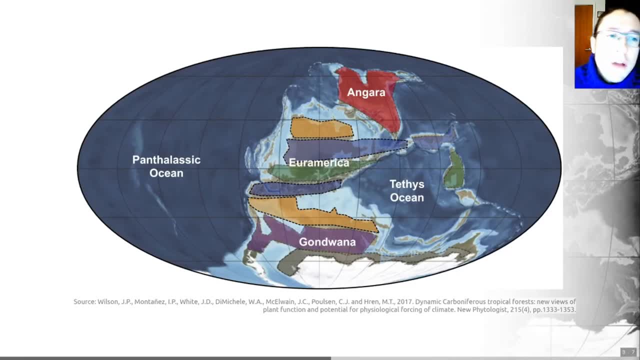 but this shifted into more provincial groupings by the mid-Paleozoic. so as we're going into the Devonian and the Carboniferous period, More widespread faunas of the early Carboniferous were succeeded, in traditionalist views, by higher degrees of endemicity during the later Carboniferous and the Permian. 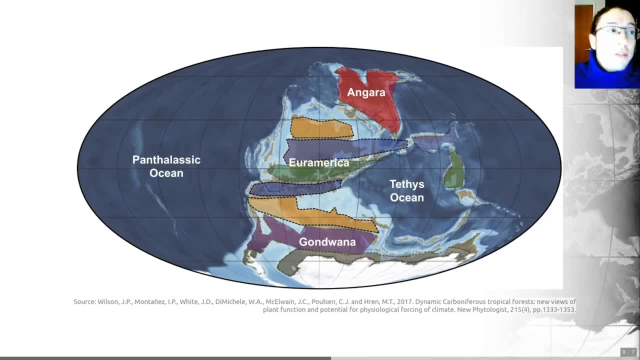 So the picture here is that you go from having this widespread set of species to more provinces, better defined provinces, as we move into the Carboniferous and Permian, And people have traditionally argued that both latitude and continental separations acted to increase this provincialism. 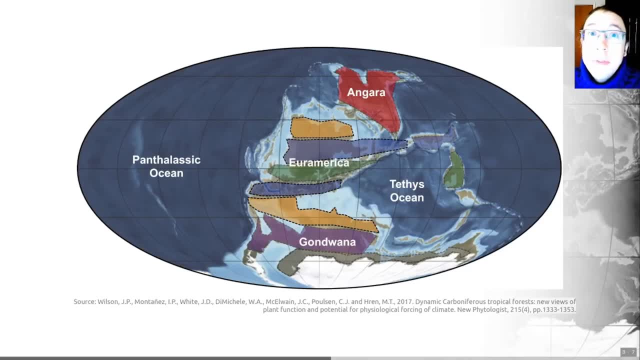 You may, though, want to compare that with the paper that I mentioned in the Paleoecology lecture by my colleague, Emma Dunner and colleagues, which actually showed the opposite using quantitative analysis. So bear in mind that many of these general patterns we've built up, 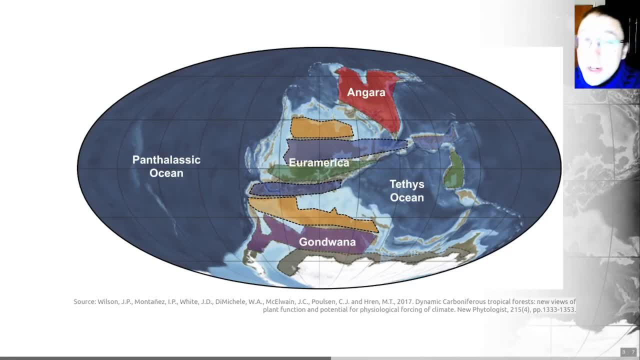 over many years and not all of them are withstanding the scrutiny of modern techniques. But we can say that floral provinces were clearly distinguishable by the Carboniferous and the Permian period. An example is shown on this slide here, and this is an upper. 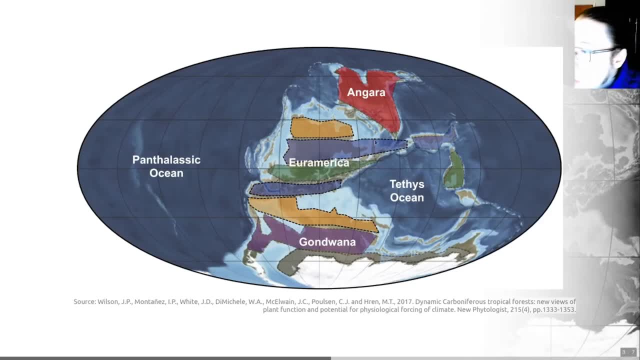 Carboniferous map for you. It shows the Carboniferous globe during a glacial phase. In the middle we've got a tropical, ever-wet forest. In the blue zones here we've got subtropical forests. These were sometimes seasonally dry. In the orange we had deserts. 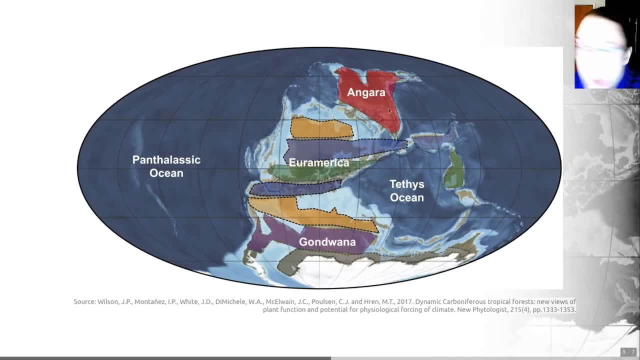 And in the red zone- you can see here- there was a temperate forest, Whereas in the purple zone, the equivalent of the south, there were southern hemisphere temperate forests. These actually differ quite significantly in the environment of the urban and the coastal around them, Just to let you know. 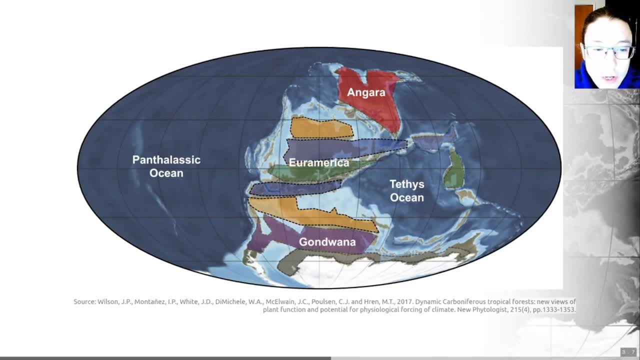 they can be used as central zones in the landscape Because they will be present throughout the winter. So there are a number of different kinds of vegetation patterns and where to find them. The grey in the bottom here is kind of like a tundra-type environment. Bear in mind that this is based on this really cool paper from 2017.. You may well want to check out, And the authors of this highlight that all of this, this broad picture of different distributions, is overprinted and strongly influenced by both topography and climate, including oceanic brat. 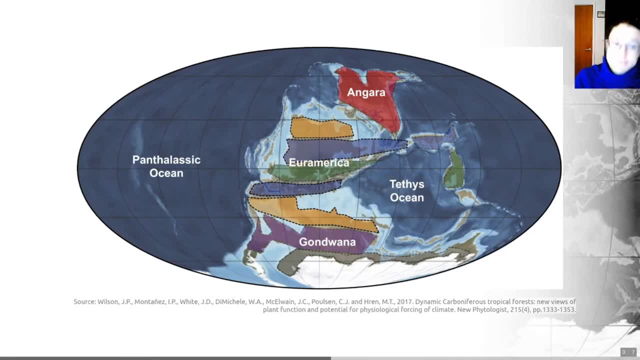 And the authors of this highlight that all of this kind of broad picture of different distributions is overprinted and strongly influenced by both topography and climate, including oceanic brat, a graphic sorry influences. so do bear in mind that's a general picture, that there's quite a. 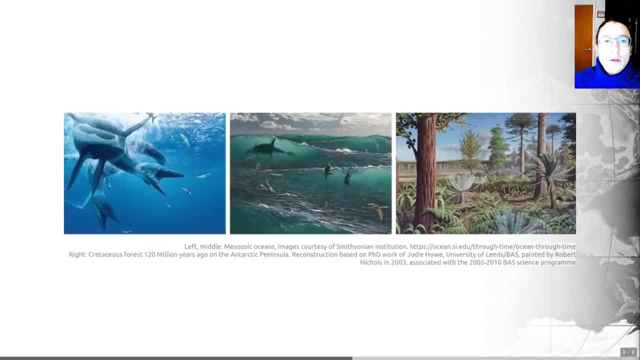 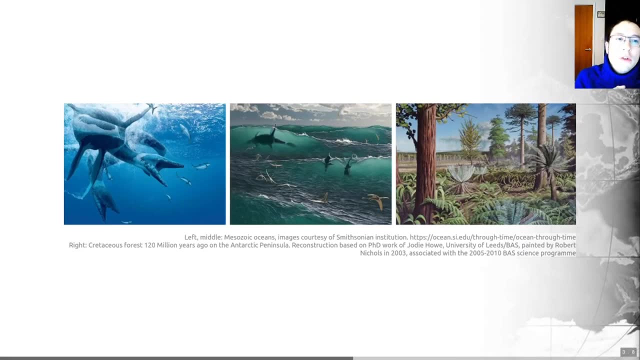 lot of nuance to it. Throughout the Mesozoic, we can say that marine faunas generally had simple patterns of high latitude and low latitude provinces, with occasionally significant local variation. During this time period, terrestrial faunas and floras, ie those on land, started off. 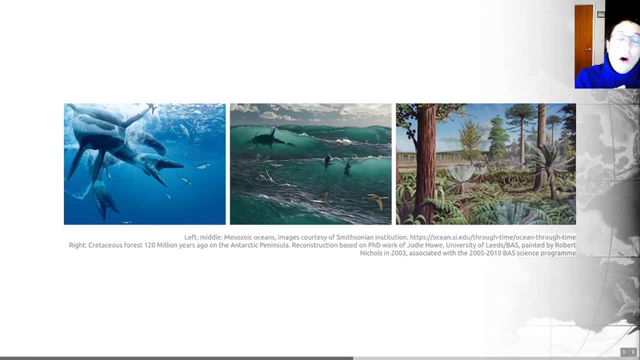 recovering from the Permian Triassic extinctions and in as part of that discovery- that discovery, that recovery, sorry, the land fauna developed provinces. During the Jurassic provinces stabilized on land and then the sea's ecosystems reached their kind of full complexity of recovery. after the Pt extinction. On land the provinces that we see were dominated by dinosaurs. 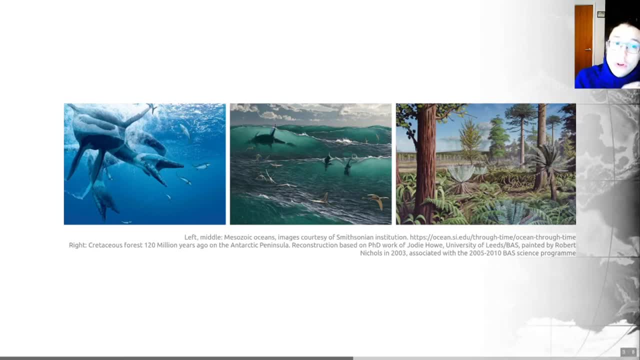 and in the ocean provinces were defined by ammonites and a variety of marine reptiles, such as the fantastic reconstructions that I've shown on the left hand side and in the middle here. The rise of the flowering plants during the Cretaceous period provided an additional provincial signal towards 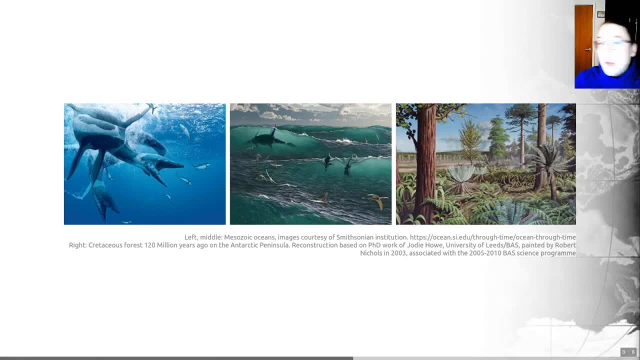 the later the end of the Mesozoic. On the right hand side you can see an example of an Antarctic forest from about 120 million years ago, And the same is true of the widespread faunas of the Chalk Sea. so we can kind of see these.